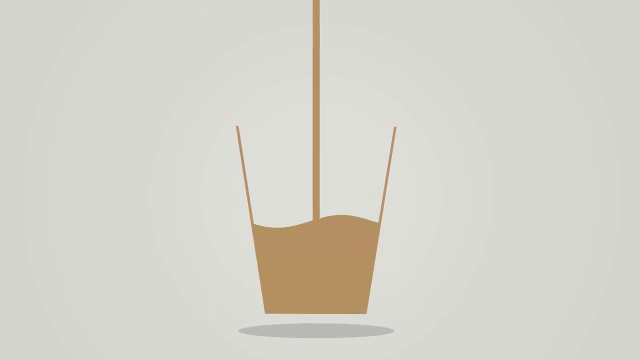 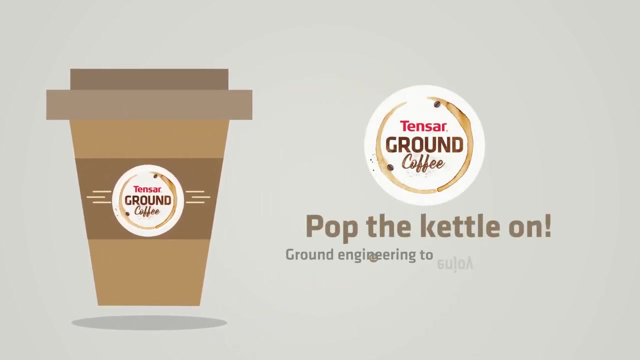 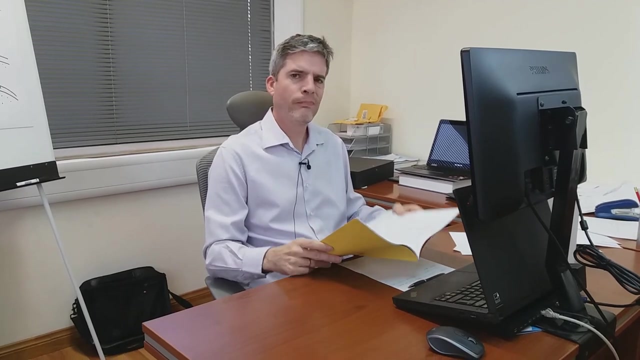 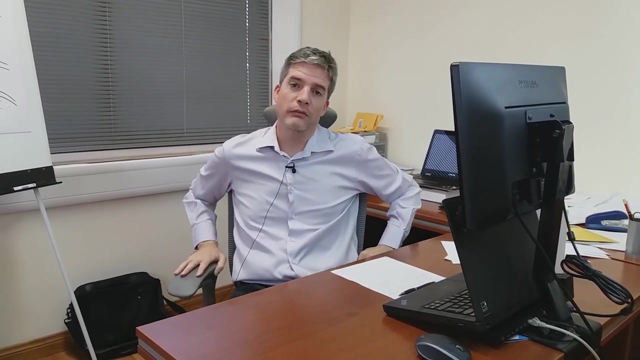 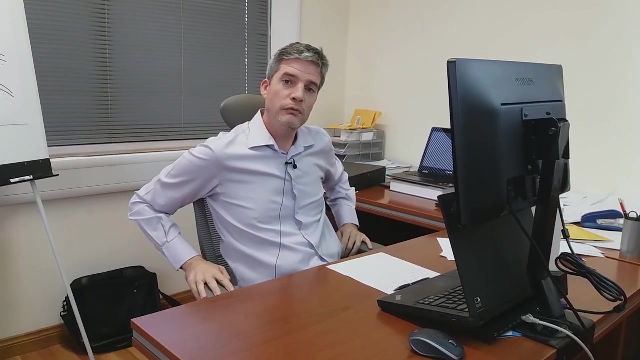 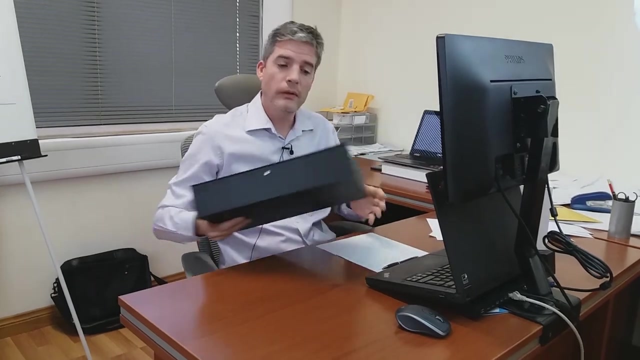 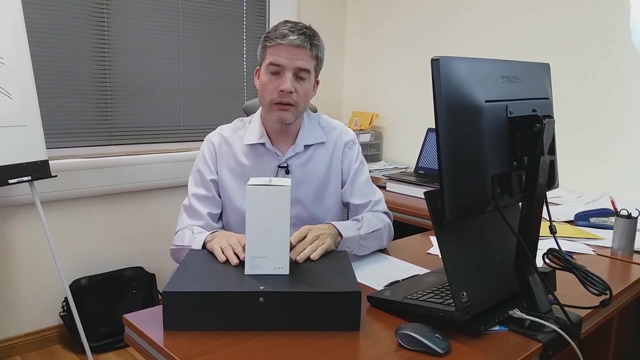 Hello and welcome to Tensar Ground Coffee. A few minutes on ground engineering to enjoy while having your coffee. This time I'd like to talk about the stabilized gravel raft solution to mitigate differential settlements resulting from liquefaction. So if you imagine that this is a liquefiable soil and we have a building on here, 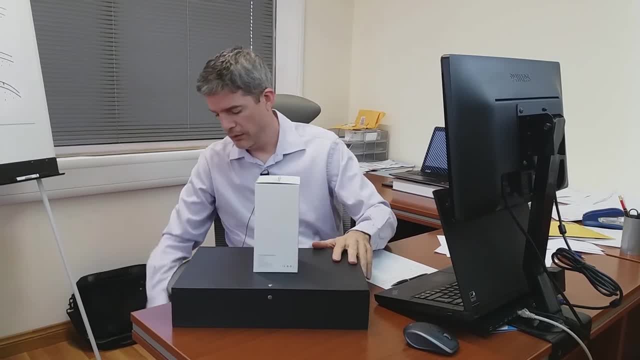 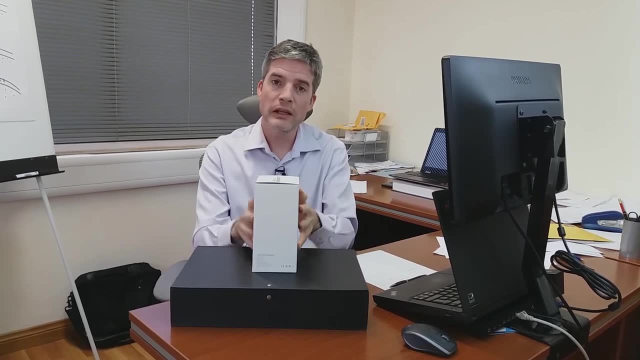 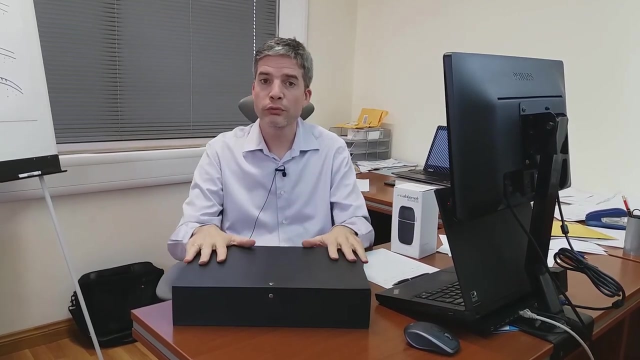 constructed on the liquefied, the liquefiable ground. Now, the traditional design methods for estimating the settlement of this building caused by liquefaction does not actually consider the building at all. It is a method called free field settlement. So, following the earthquake and 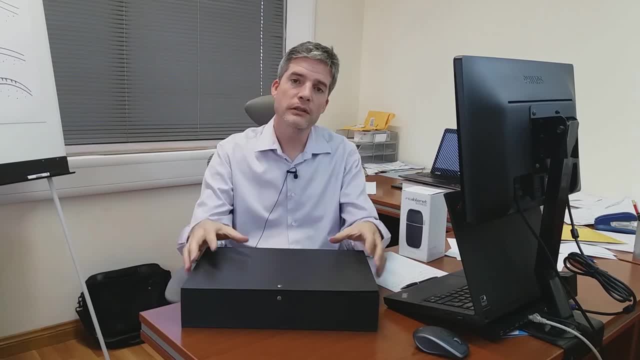 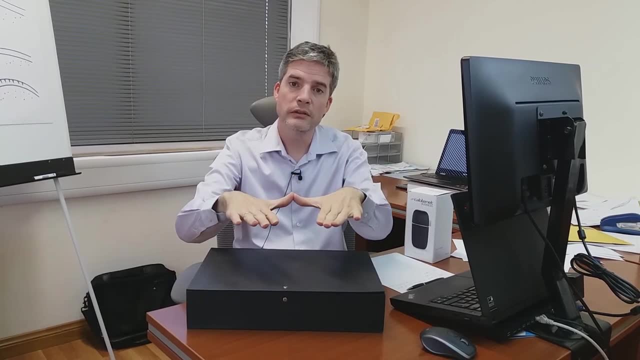 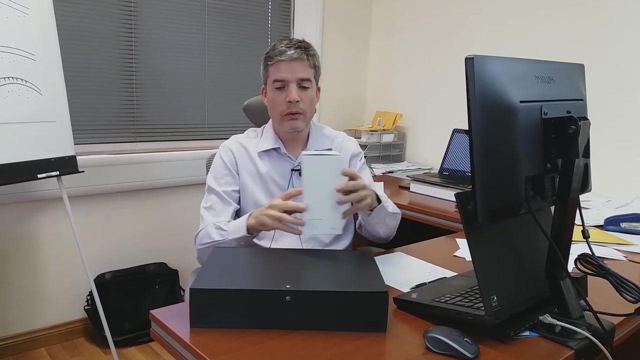 liquefaction. when excess pore pressures have been generated in the liquefiable ground, those excess pore pressures dissipate and the ground surface settles. and it is just assumed to be a uniform settlement like that, But the latest research has shown that a lot of the settlement occurs during the earthquake. 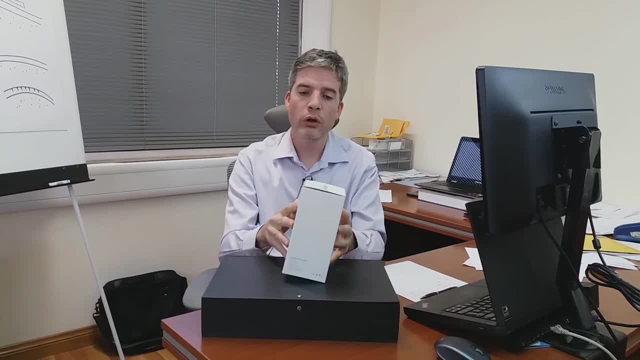 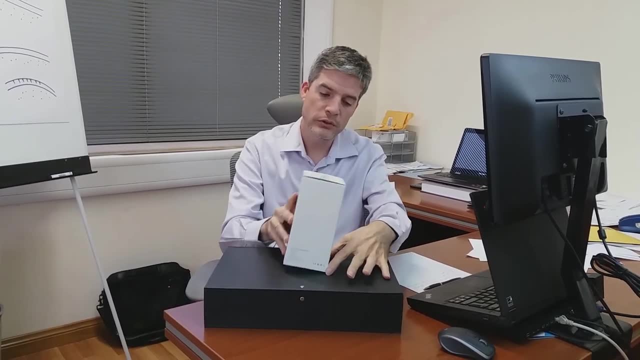 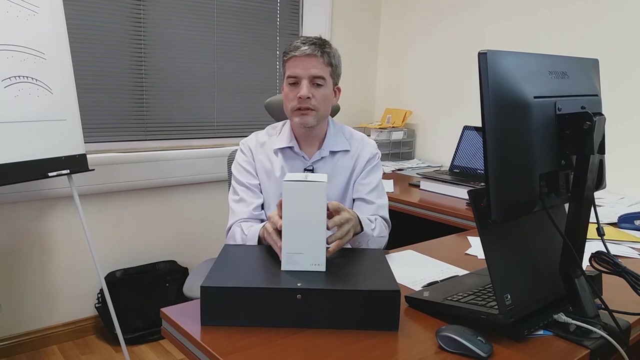 motion. So during an earthquake the building will rock from side to side and if this ground has liquefied, we're getting bearing capacity failure and shear induced settlement on each side. So most of the settlement accumulates this way and we actually get differential settlement and curvature of the 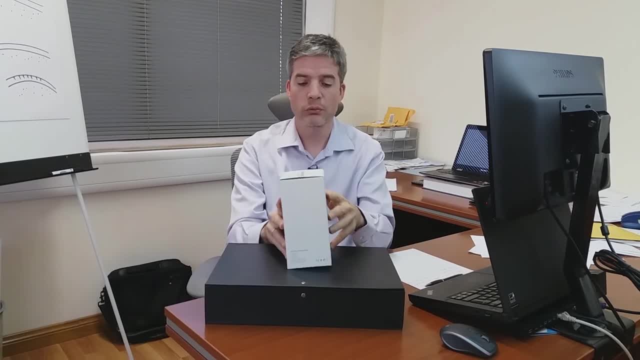 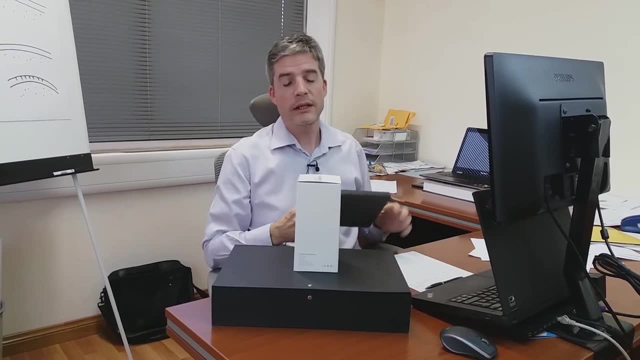 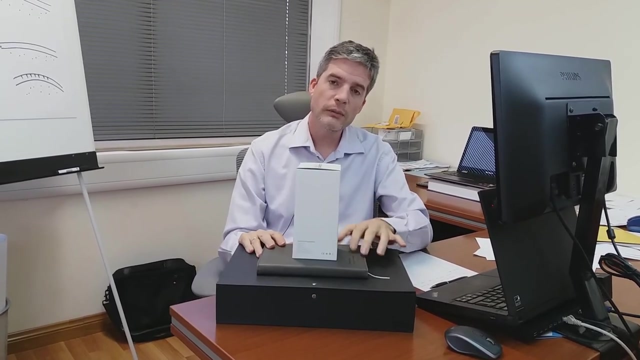 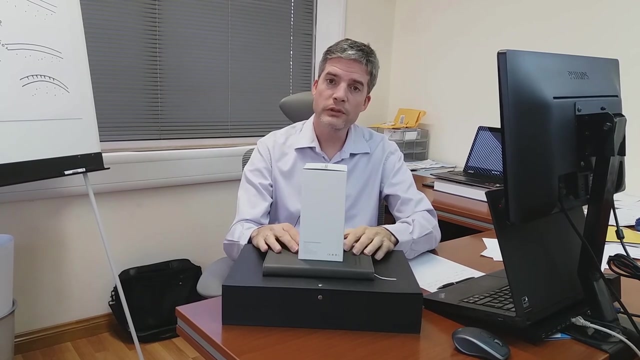 foundation, which is what really causes the damage from this rocking. Now the stabilized gravel raft solution mitigates that settlement and there were a few cases in Christchurch, New Zealand, where a stabilized gravel rafts were installed prior to the earthquakes. So we have some case studies which demonstrate remarkable performance of these. 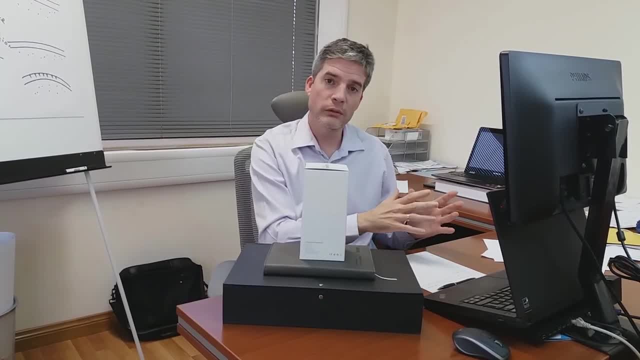 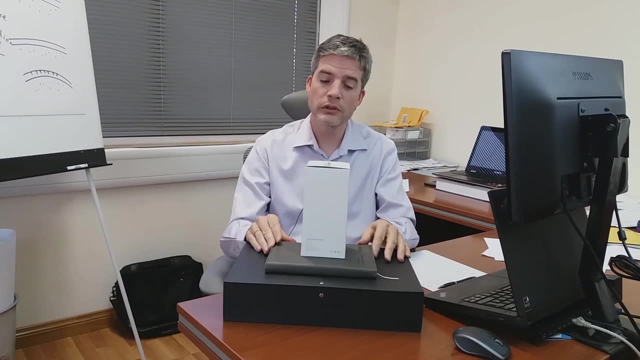 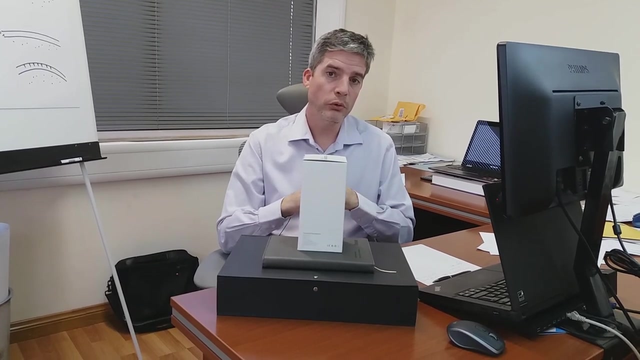 stabilized gravel rafts compared with areas just off the raft and also in the Charlotte Was 같이 Great the investigation trials afterwards. using explosive induced liquefaction they tried out different ground improvement methods and a stabilized gravel raft performed very well in those as well. So how it works is you have a granular material.